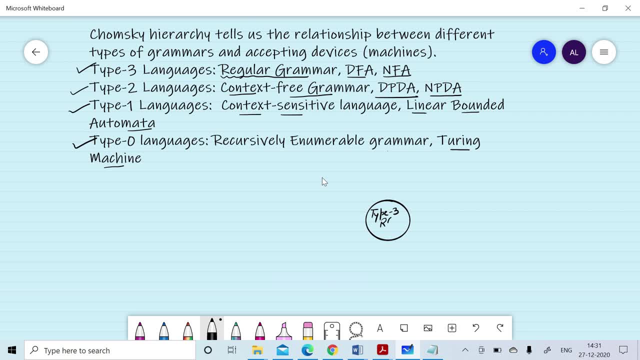 we can able to design regular grammar. we can able to write down regular expression. we can able to design NFA As well as we can able to design DFA. The next type of language is type 2 language. We will also call it as context-free languages. Corresponding to it, we can able to write down: 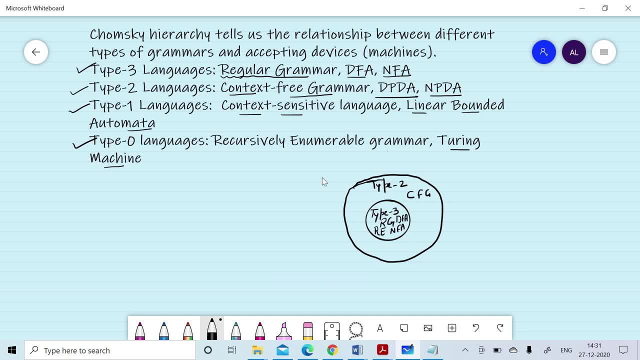 CFG. that is context-free grammar and we can able to design Deterministic PDA as well as Non-Deterministic PDA. But Non-Deterministic PDA is more powerful as compared to Deterministic PDA, So we can able to design Deterministic PDA. 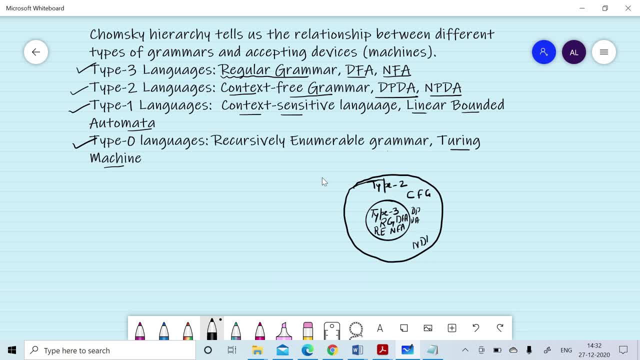 And we can able to design non-deterministic PDF. If we will consider the language, L is ANBN. it is a context-free language. We can able to design deterministic PDF for it, but we cannot able to design regular grammar for it. 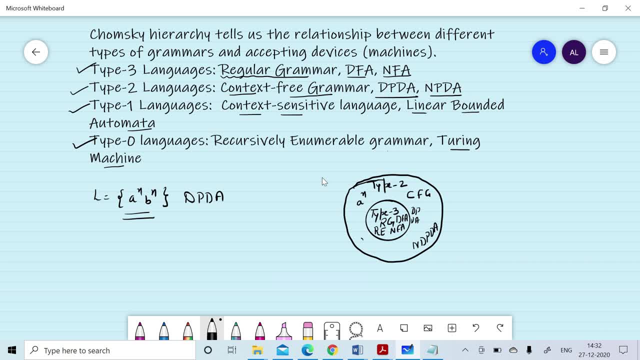 We can have language ANBN, which is context-free, but not a regular language. Similarly, we have another language: L is odd palindrome over A and B. We can able to design non-deterministic PDF for it and we cannot able to design deterministic PDF for it. 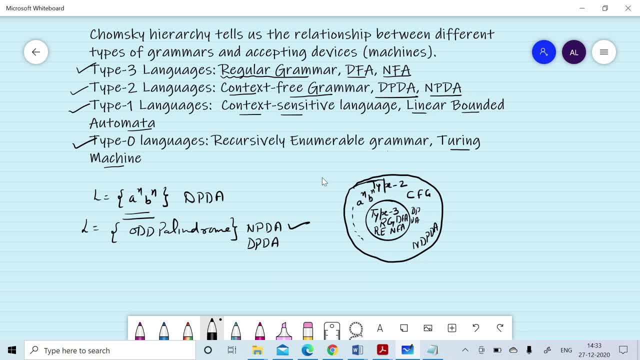 So non-deterministic PDF is more powerful, So we can call it as it can be further divided into two parts: One is corresponding to which we can able to design deterministic PDF, and one is corresponding to that we can able to design non-deterministic PDF. 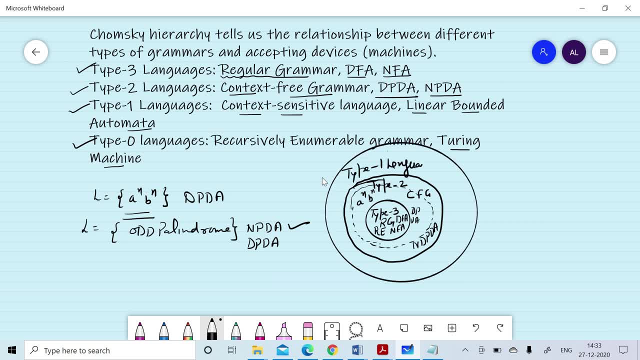 The next type of language is type 1 language. Corresponding to it, we can able to design context-sensitive grammar and we can able to design linear bounded automata corresponding to type 1 languages. Last one is type 0.. Corresponding to it, we can able to design Turing machine and we can able to write down. 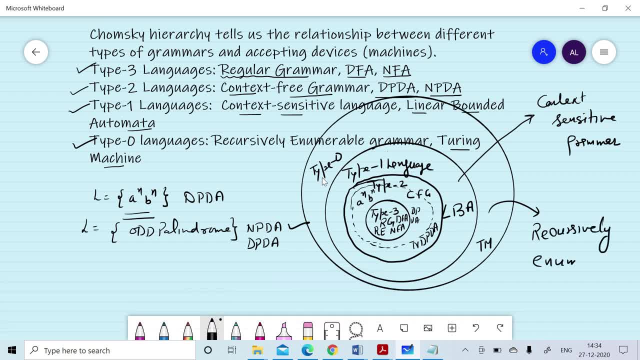 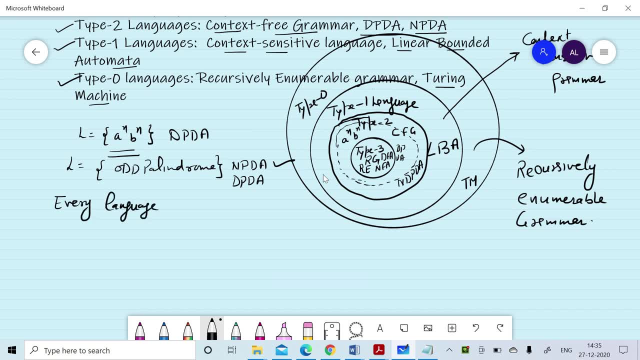 recursively enumerable grammars or unrestricted grammar- we can call it as Context-free language of type i- is by default of type i-1.. What it means, if we have any regular language, that is by default, that is context-free language, that is context-sensitive language, as well as recursively enumerable language or we 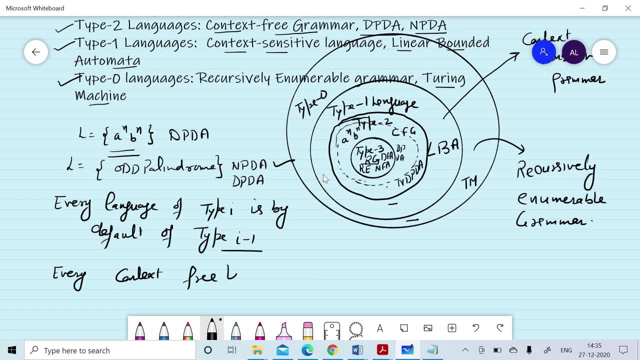 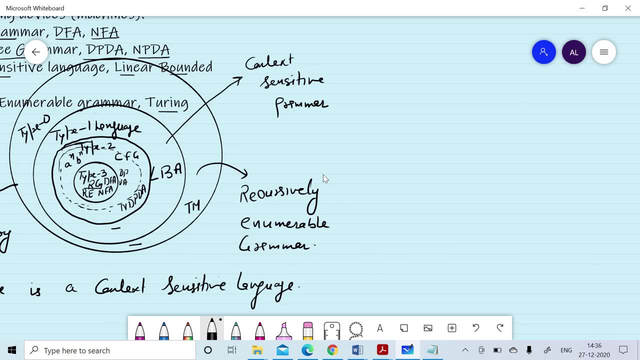 can say: every context-free language is by default, a context-sensitive language. Now we will discuss what is the meaning of linear bounded automata. A linear bounded automata, that is, LBA, can be defined as a non-deterministic Turing machine which only use the input tape space c1 multiplied by length of the string. 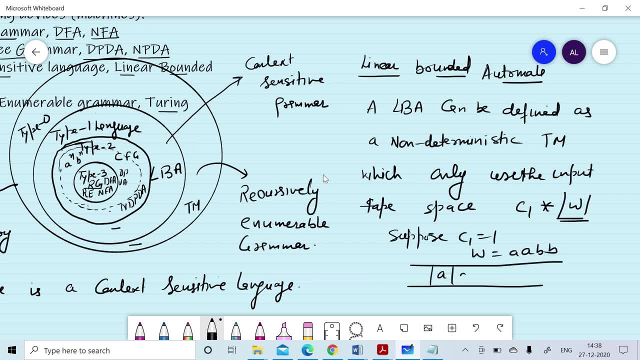 wo small. we have c1 has one. so we have the wo as aabb. so we have the left and right marker. that is denoting the left marker of the input tape and right marker of the input tape. we cannot able to read this left marker. 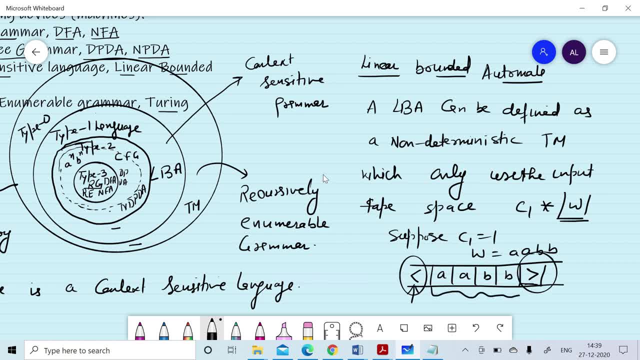 as the length of machine, though we could impossible. why, since we don't have- and well as- the right marker, we have to only utilize this much space for processing of linear bounded automata. so linear bounded automata is acting as a turing machine, but we have the foundation. 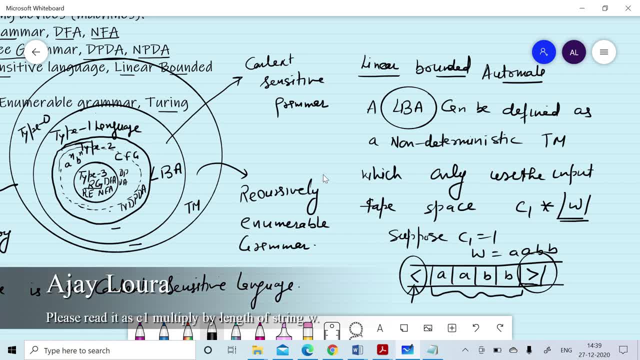 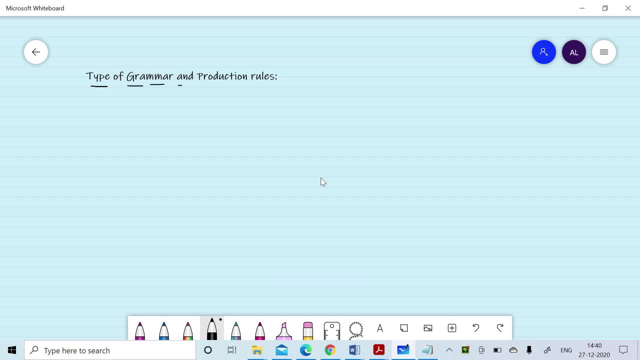 of the space that is given by c1 multiplied length of input tape. now we will discuss what are various kind of restriction on different type of grammars. so initially we have type 3 language or regular language. we are defining regular grammar corresponding to it and regular grammar can be classified as left linear or right linear grammar. linear means: 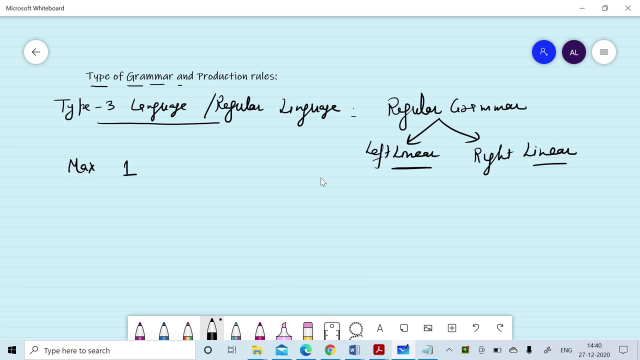 maximum one non-terminal is allowed in the right hand side of a production rule. if it is extreme left, then we are calling it as left linear. if that single non-terminal appear in the right most position in all production rule then we will call it as right linear grammar. in the left hand side of all production rules only one non-terminal is allowed. 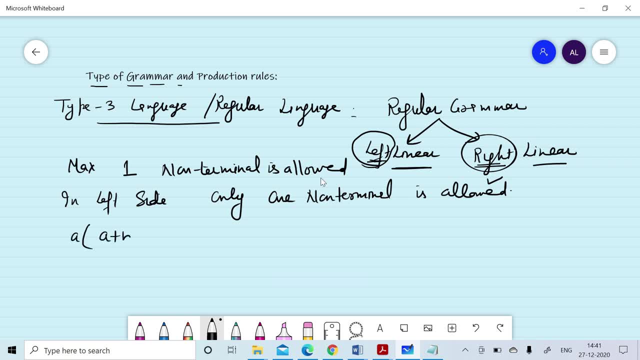 for example, suppose we want to design right linear grammar that is starting with a and ending with b, so we can design it as: s will give you a, a, only one, a. we want to generate a and then, using the capital a, we want to generate a number of a and b. so we will generate it by a, a, b, a or b. 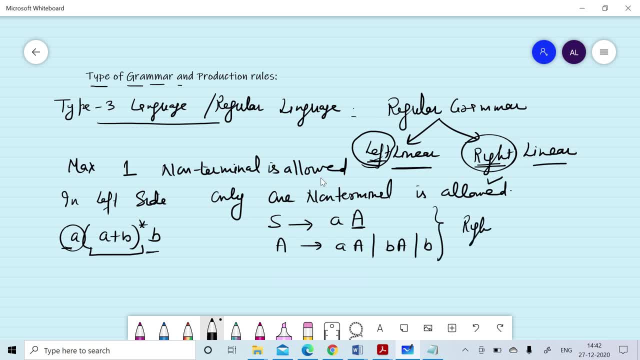 we will call these kind of rules as right linear, because in the right hand direction maximum one non-terminal is presenting and that non-terminal is appearing at the extreme right position. in the left hand side, only a single non-terminal is allowed if we want to design left linear grammar. 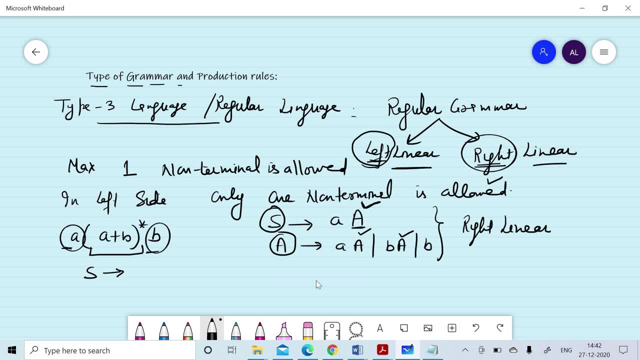 can design it as like this one: We will generate the first symbol as B, so A, B, and using A we will generate a number of A and B, so A, A, A B, and it is replaced by A or terminated by A. So again, maximum one non-terminal is allowed in the right hand side and that is appearing at extreme left. 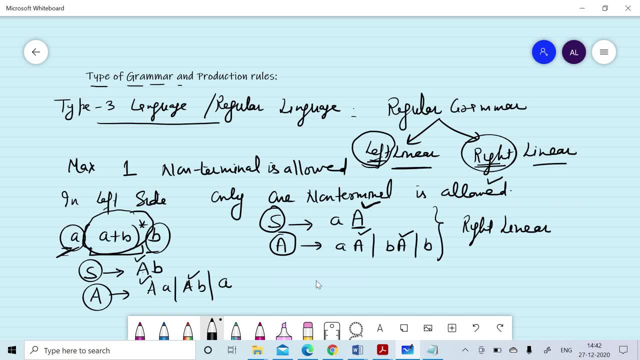 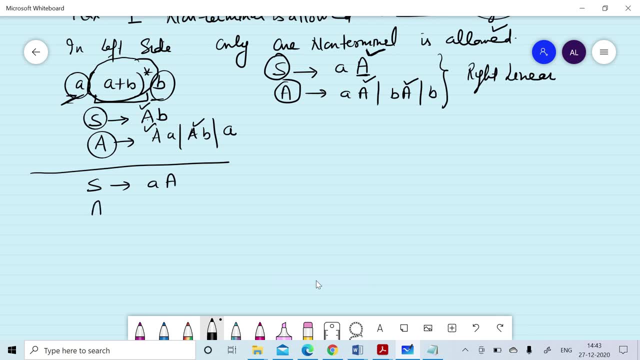 position and in the left hand side only a single non-terminal is allowed. Now consider the production rule: S will give you A, A, A will give you S, B and S can give you null. also, It represents the language. L is A, N, B, N and which is a context free language. This is not a left, linear or right. 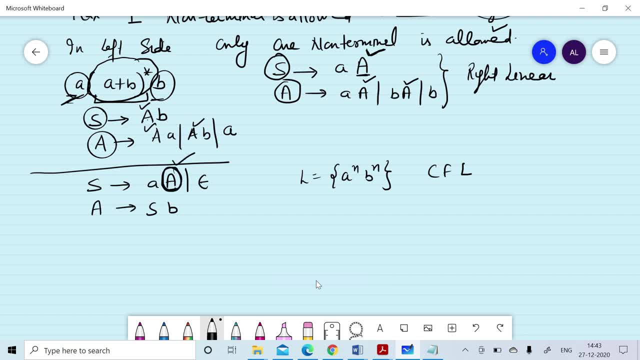 linear language, because in this production rule A is appearing at extreme right position in the left hand side, So again, maximum one non-terminal is allowed, and in the left hand side this production S is appearing at extreme left position. So these production rule are neither left linear nor right linear. So this is not a regular grammar. For a grammar to be regular, it: 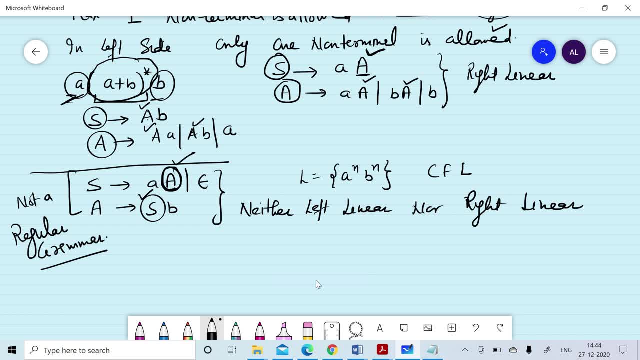 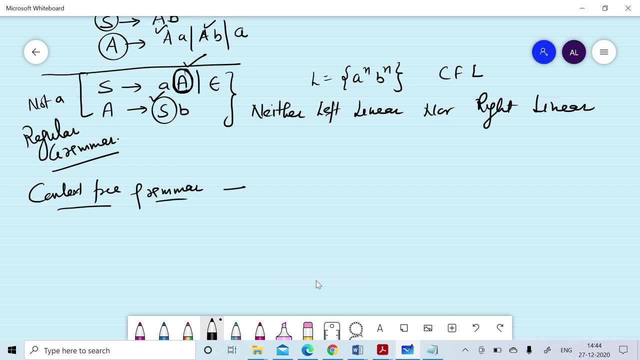 is either left linear or it is right linear. Now we will discuss context free grammar. In a context free grammar, only one non-terminal is allowed in left hand side of every production rule. There is no restriction in the right hand side. So it will be of the form A, will give you alpha. 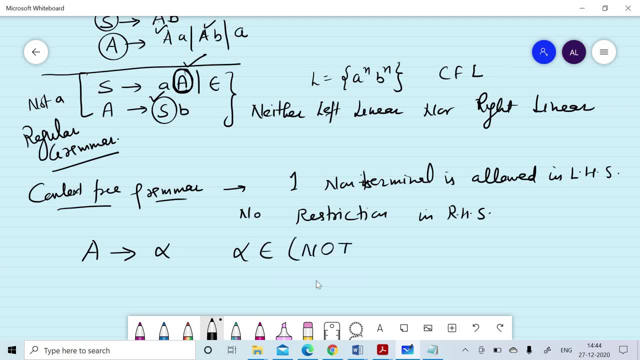 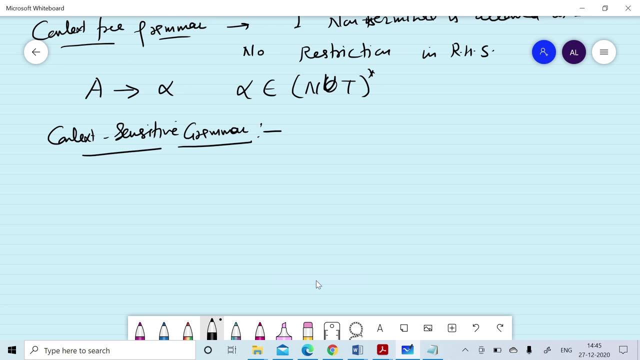 and alpha is any string over terminal and non-terminal. So the given grammar is a context free grammar because in the left hand side we have only a single non-terminal. In the right hand side we have no restriction In context sensitive grammar. we can have any combination of: 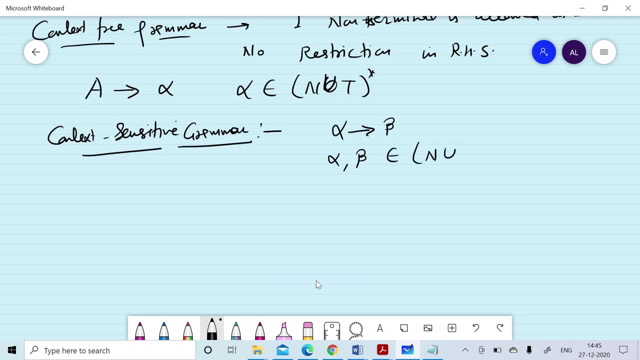 terminal and non-terminal, In the left as well as in the right hand side, But the length of alpha must be less than equal to length of beta. What it means? we have these kind of rules because length of left hand side is 2, length of right hand side is also 2, but we cannot allow these kind of rules. 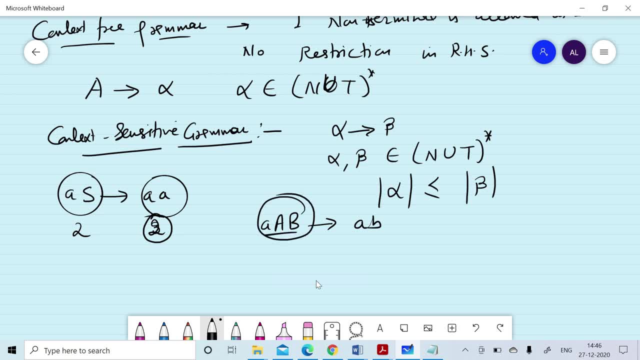 because length of alpha in the left hand side is 2. we cannot have these kinds of rules because length left hand side is 3, length of beta in the right hand side is 2.. We can have any number of terminal and non terminal in the left as well as in the right hand. 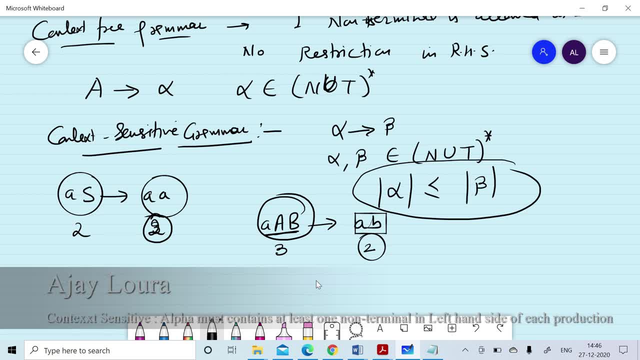 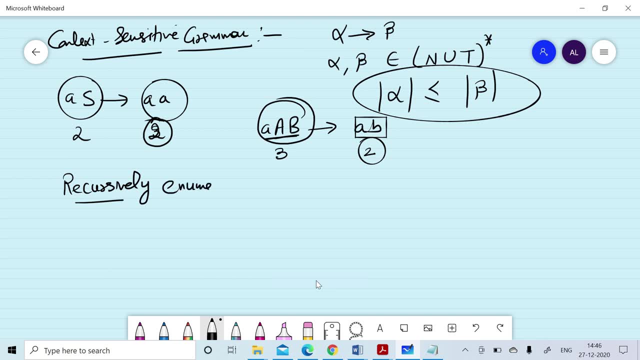 direction, but the condition must be satisfied that the length of alpha is less than equal to length of beta. Now we will discuss the case of recursive enumerable grammar. It is also known as type 0 grammar, and in type 0 grammar we have no restriction on alpha and beta, Only one point. we should note that alpha 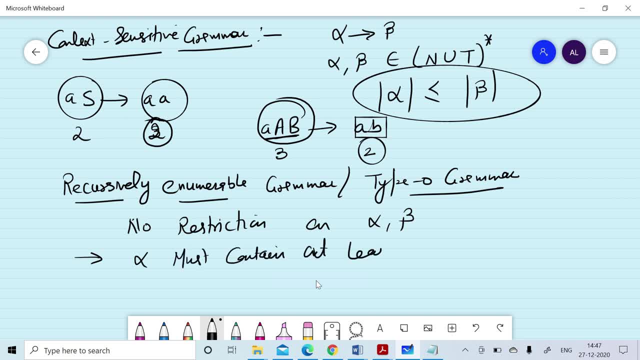 must contain at least one non terminal. In the next session we will discuss few example for identifying the type of grammars. Thanks for watching this session.